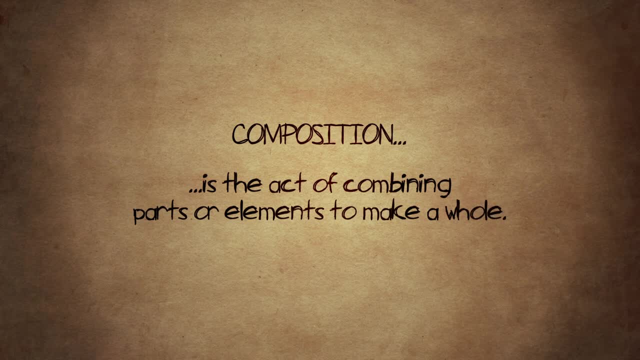 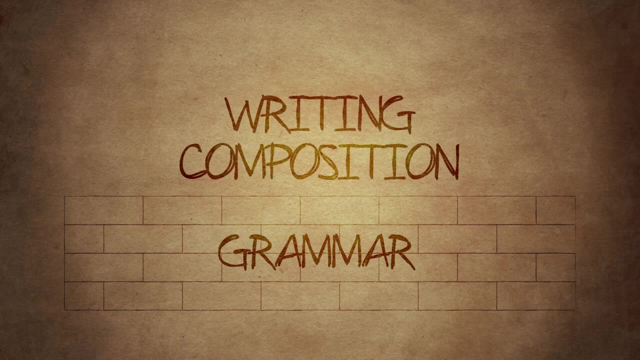 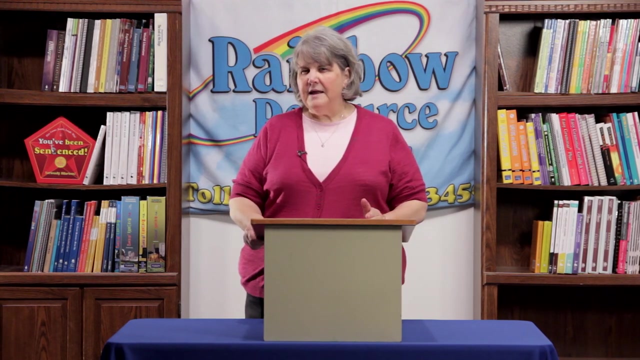 is the act of combining parts or elements to make a whole. Like phonics, provides the building blocks of reading, grammar provides the building blocks of composition or writing And it ultimately gives us the strength of structure to yield beautiful collections of words that convey thoughts and ideas and emotions. But grammar is just a starting place. How? 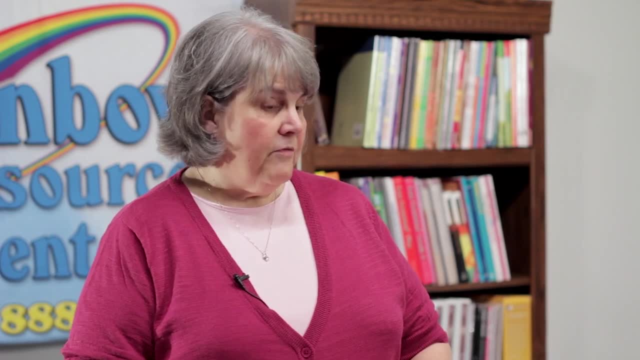 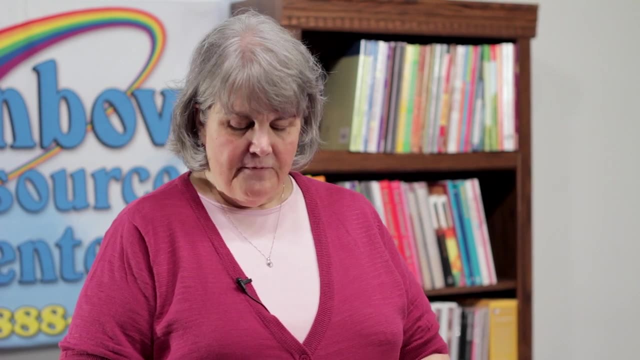 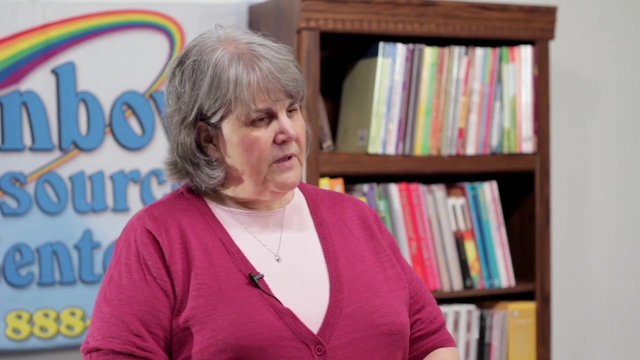 thoughts and ideas are combined and organized is another part of writing And, of course, also important are the stylistic elements that make it enjoyable to read, or the clarity to follow the author's thoughts, Or the involvement to care about what's been written. There is a sequence to producing. 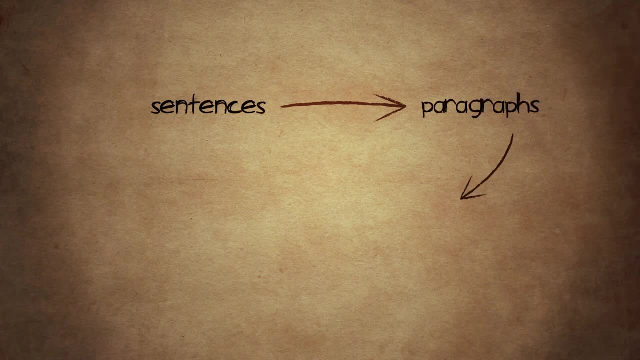 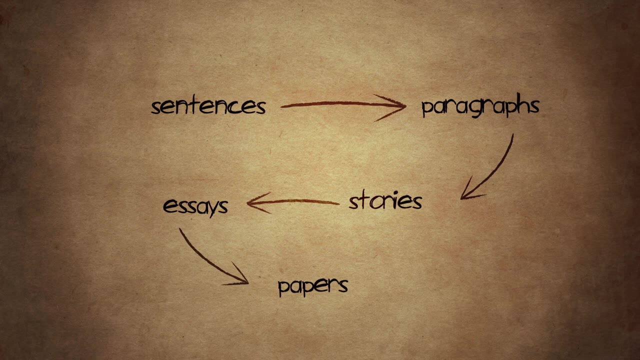 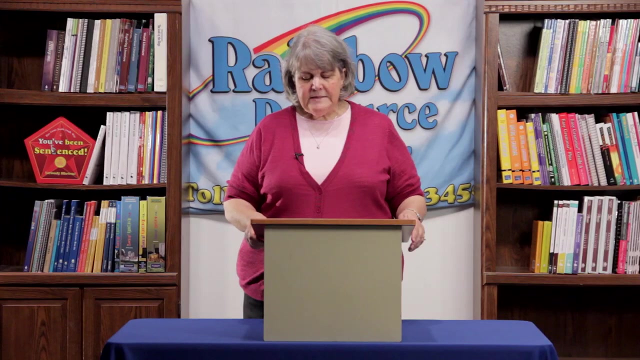 good writing: Composing sentences, then paragraphs, then stories and essays and papers. Children need to understand the parts in order to put the whole thing together properly, But they also need experience with good examples and practice with the process. A similar sequence of skills leads to effective speech, Just like in composing an essay or 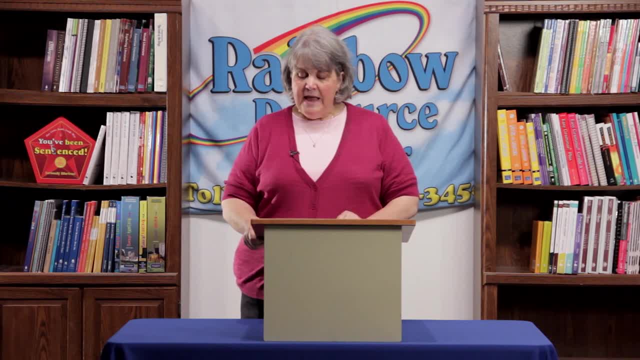 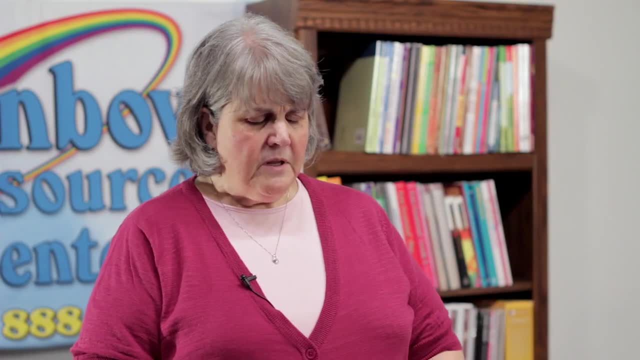 a story speech takes the same building blocks and adds in the elements of appeal to auditory learners, Voice quality, drama theatrics. I won't spend a lot of time on this one, but I do want to note that public speaking is the number one fear of Americans There. 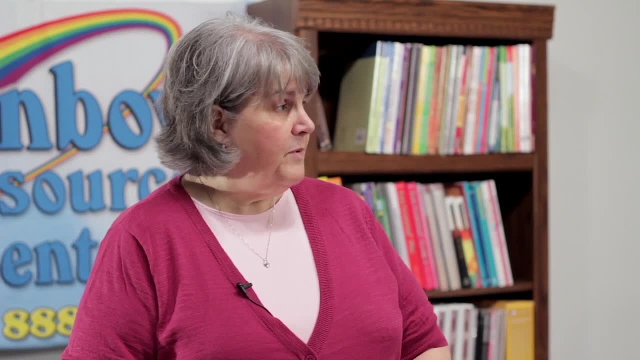 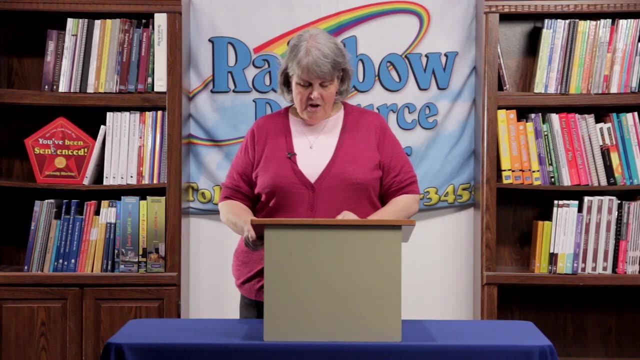 are very few people who really enjoy speaking in front of a large group of people. Teach your children to overcome this fear and they will be a step ahead of many adults. Earlier. I compared vocabulary to a golden thread. I used to say I'm not going to be able to. 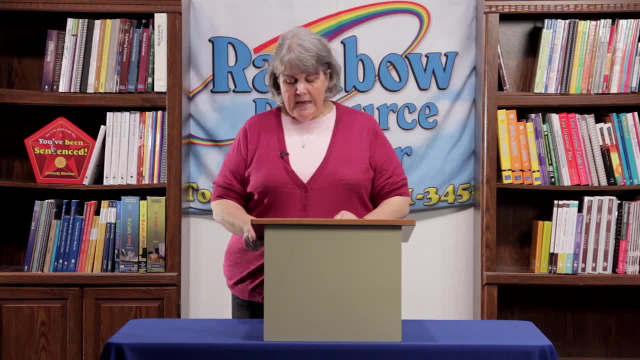 speak in front of a large group of people. I'm not going to be able to speak in front of a large group of students. We don't have to worry about that. In order to improve vocabulary, words and sentences and texts need to be in keeping with the conversation. 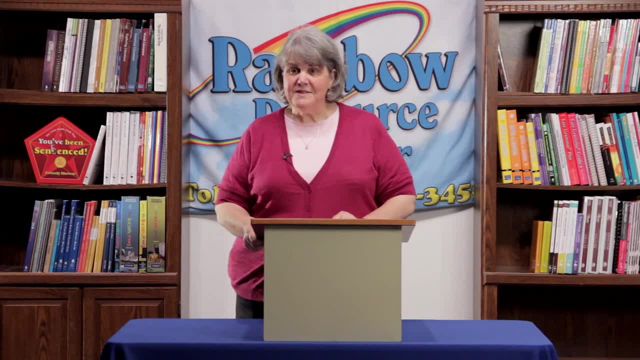 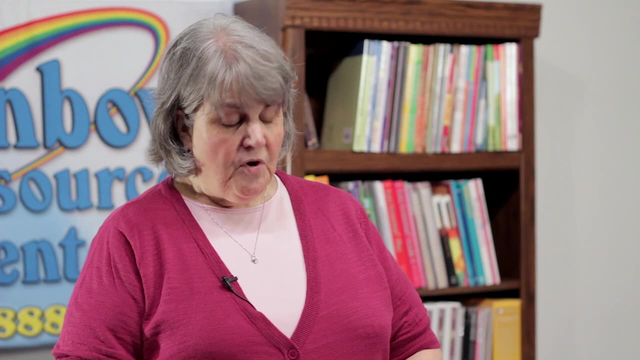 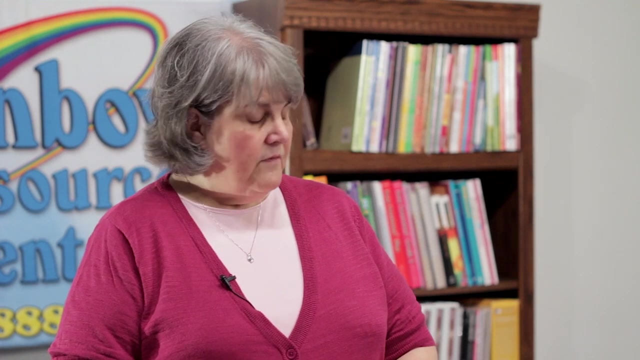 In composition. the expert use of vocabulary makes our writing more interesting and specific. When speaking, we might find our intelligence being judged by the extent of our vocabulary. Expanded vocabulary also increases a student's ability to do well on standardized testing. Strong scores on college entrance tests like ACT, SAT and even the GRE are largely dependent 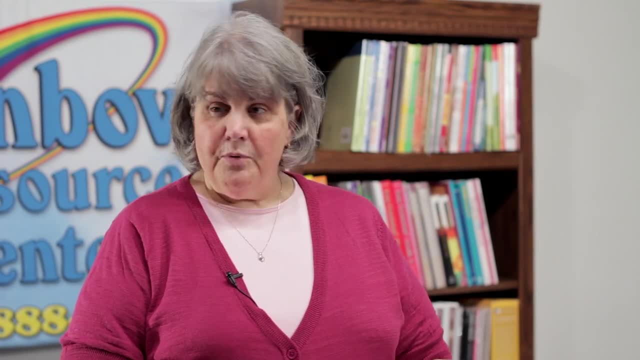 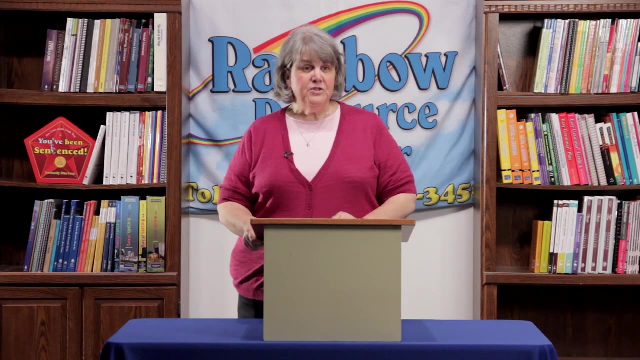 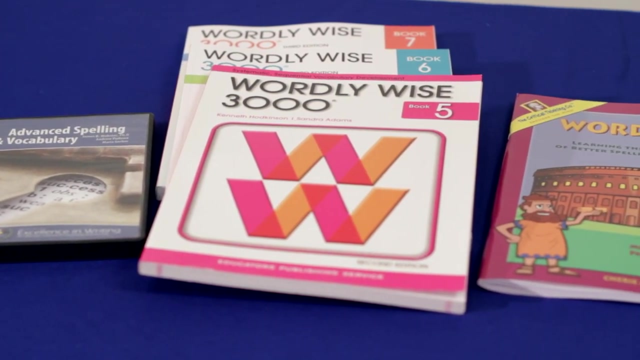 on vocabulary. Many reading and literature programs include vocabulary studies, but there are stand-alone vocab programs as well. These programs might be subject-based, like IEW's Advanced Spelling and Vocabulary, or they might be general usage-based, like Wordly Wise 3000, or they might be roots-based. 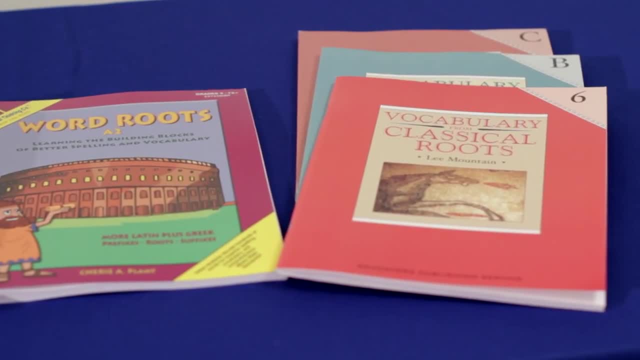 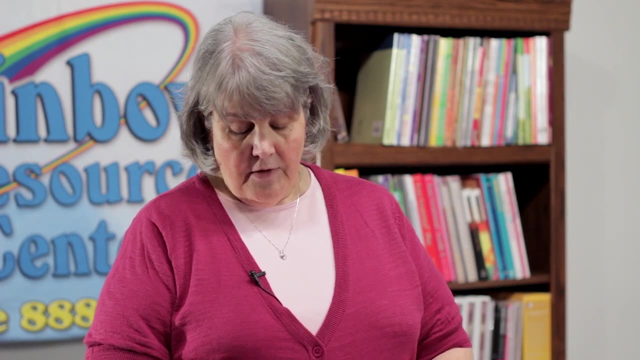 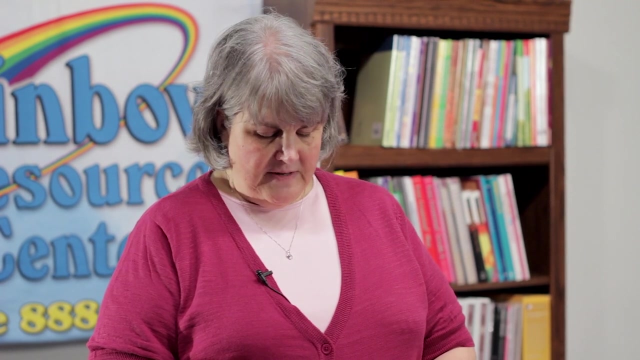 like Word Roots or Vocabulary from Classical Roots. About now you might be wondering how we ever got from reading and writing to the myriad of programs that have something or other to do with language arts. You might also be thinking: okay, so now I know a little bit about each of. 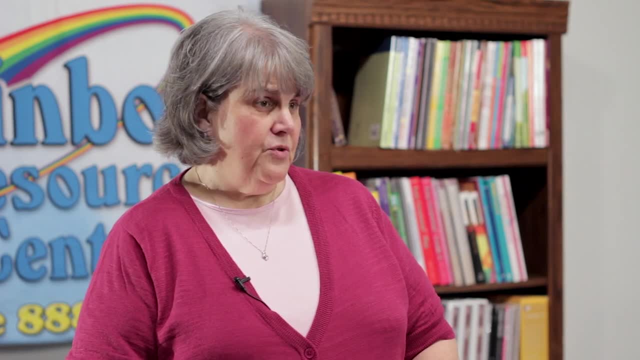 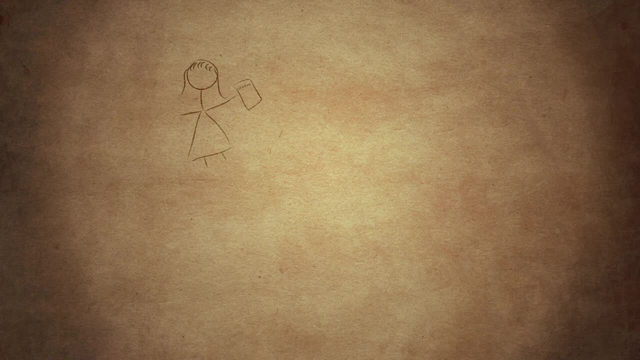 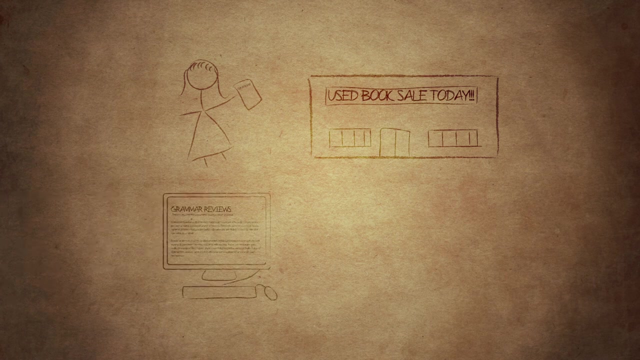 these components, but I still don't have a good idea of what I should choose. Fair enough. So how do you choose? Do you pick the one or ones your friend is using? Do you pick up something at a used curriculum fair? Do you check online reviews and see what everybody else likes? 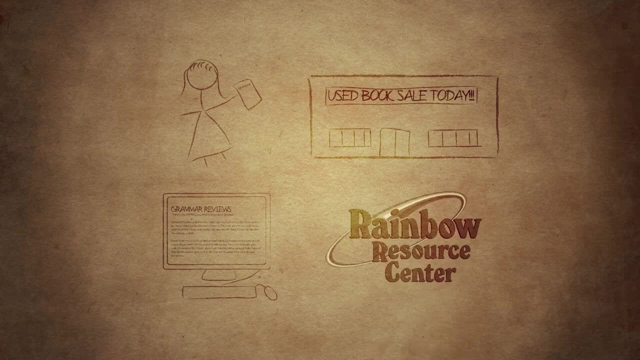 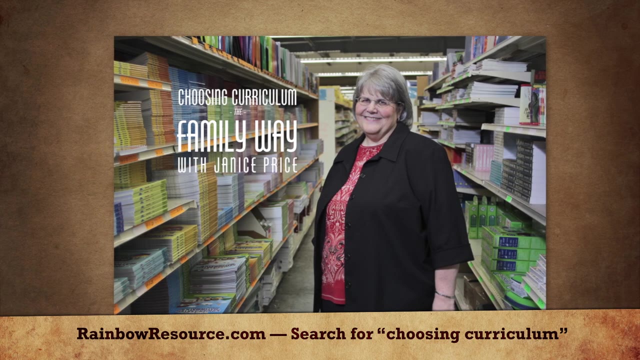 Or do you call Rainbow and ask: what are our top sellers? If you haven't already watched our Choosing Curriculum, the Family Way workshop, I'd encourage you to take a look at it and to consider the family questions posed there. These are the things that are important to consider as 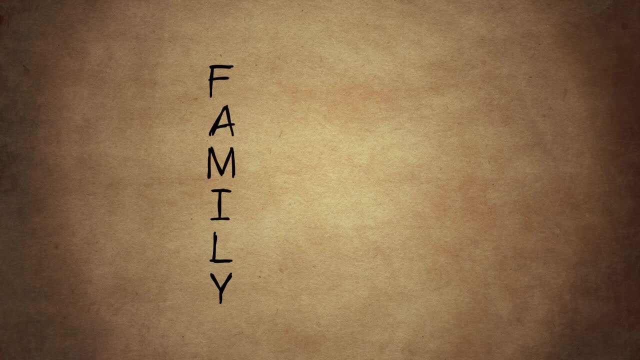 you choose curriculum and some of them might matter more to you than others do. First, is this a faith-based product? The F in our family acronym is for faith. Two, what is the predominant homeschooling approach of this product? The A is for approach. Three, how much money does it cost? Is it a good value? Does it fit in our 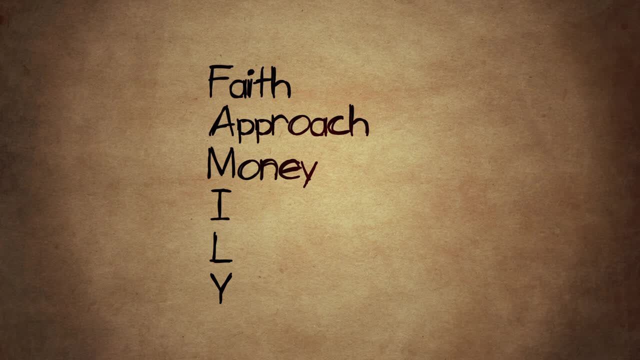 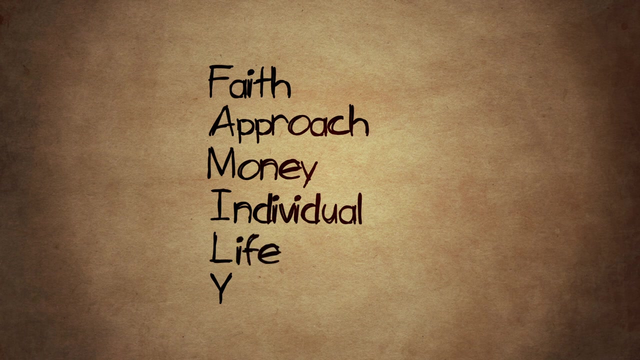 budget. Is there a less expensive way to accomplish the same thing? M is for money. Four: how will the individuals in my family with their distinctive learning styles, respond to this program? I is for individual. Five: how will it work with the other aspects of my life? L is for life And six does the? 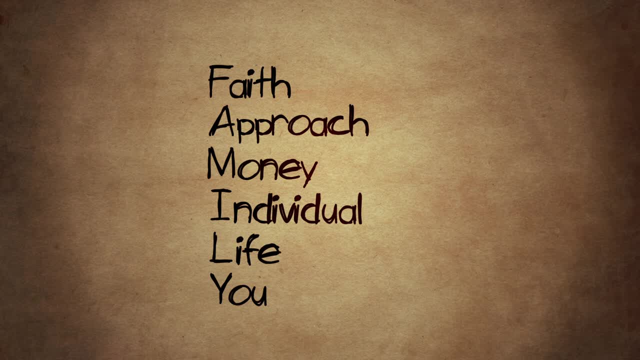 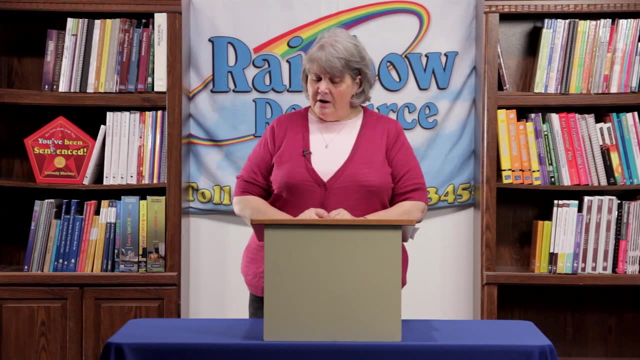 program. give me what I need to teach this subject? Y is for you. Any one of these questions might be the most important one for you, but in terms of language arts curriculum, I tend to think that it is the teaching approach that makes the most. 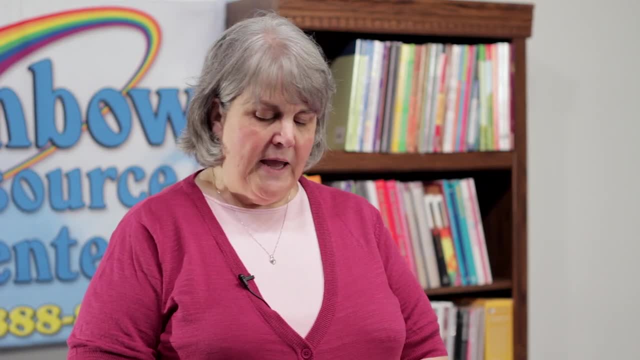 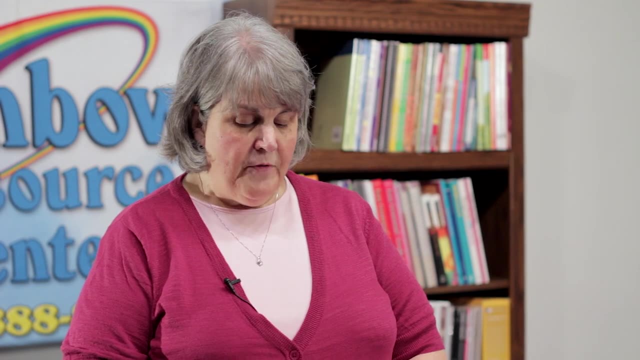 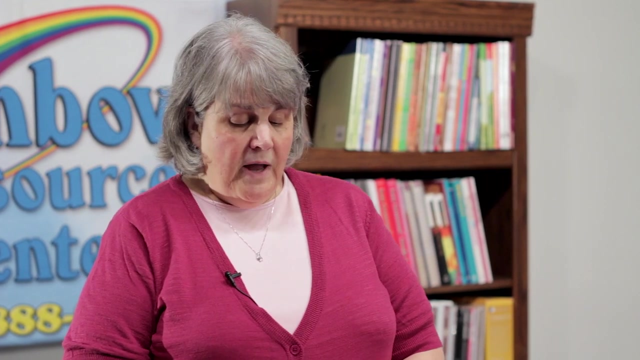 difference. Educators have been discussing, arguing actually for years over the role of grammar or the need for diagramming, or when to start teaching grammar, or whether to emphasize free writing without corrections, or formula writing or learning from models. Frankly, we're not likely, you're not. 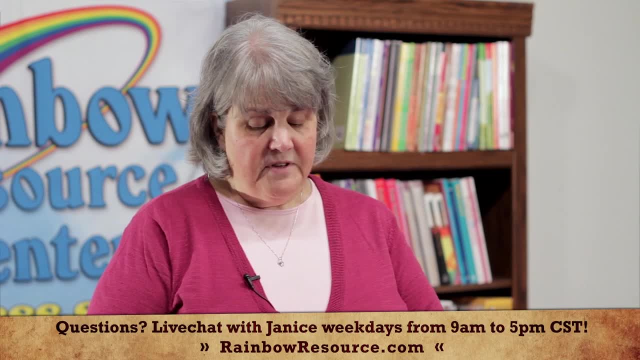 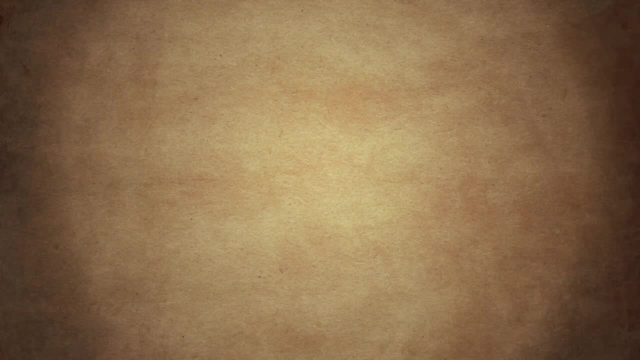 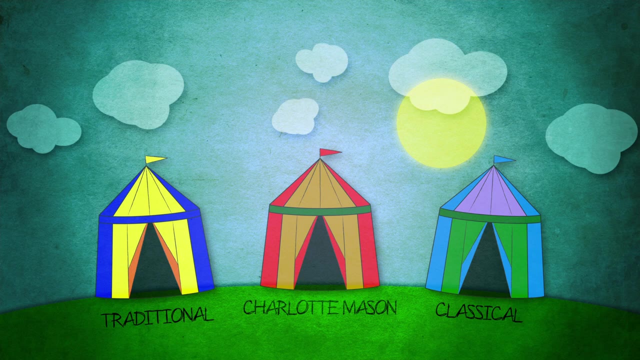 likely to solve any of these dilemmas, but you do need to have some idea of what you think is important And you need to choose a curriculum that is consistent with your thoughts. Most of our language arts curriculum choices fall into three different camps: Traditional, Charlotte, Mason or classical. And, of course, there are 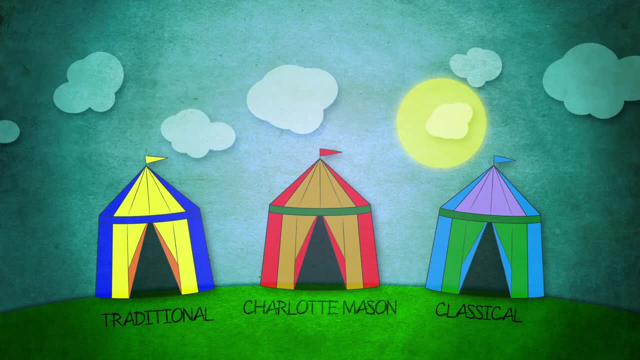 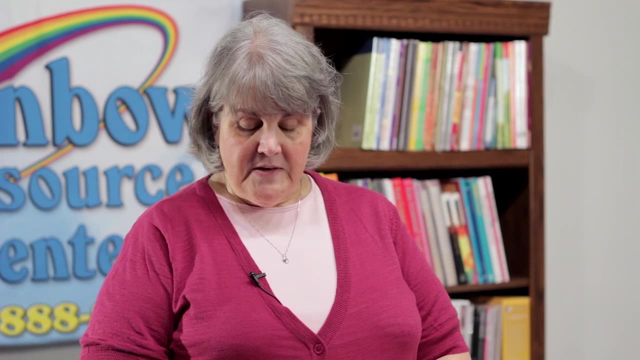 variations and blendings of these as well. Traditional is what you probably had when you were in school. There is a teacher edition and student text or workbook. A lesson is taught by the teacher, the student follows along and then there's an assignment to reinforce the concept followed. 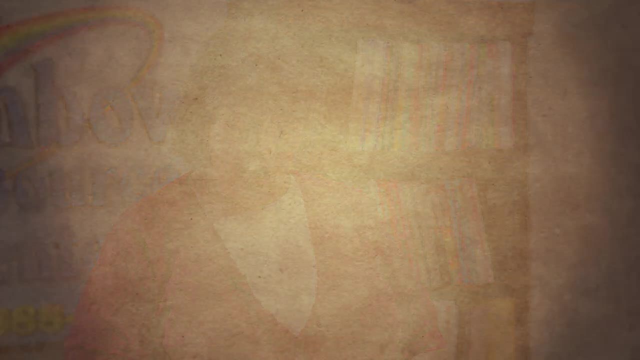 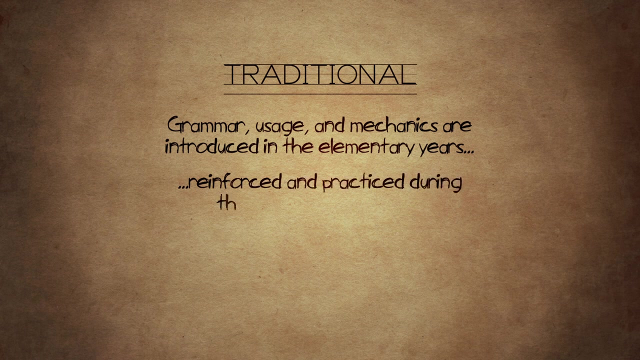 by tests to make sure you learned what you were supposed to learn. Traditional courses tend to introduce grammar usage and mechanics in the early elementary years, hit them pretty hard with depth and determination in the middle school years and expect proficiency at the high school level. Composition is handled in much the same way, usually in alternating. 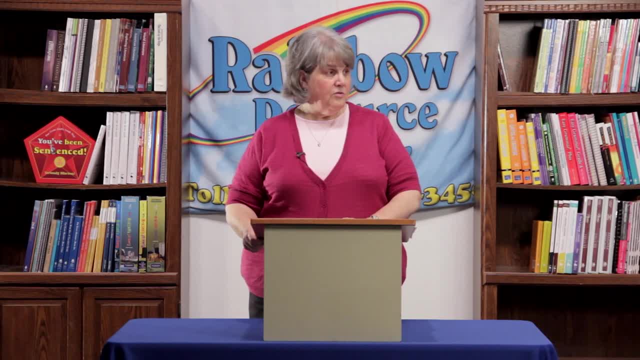 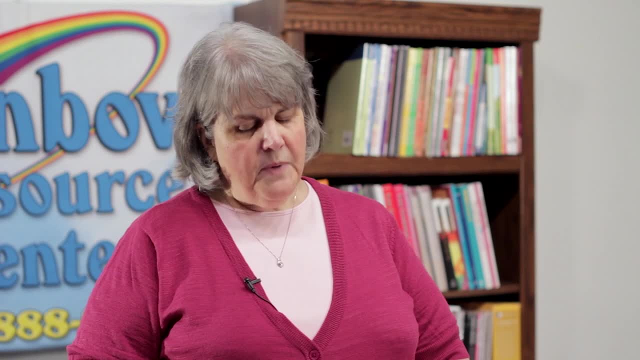 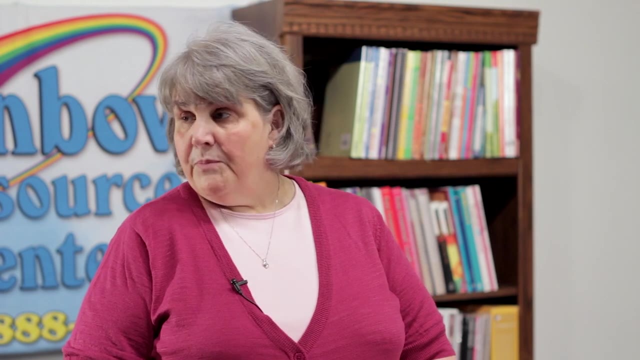 chapters or sections of the text and with systematic instruction, In other words, first sentences, then paragraphs, then stories and essays. Traditional publishers are also likely to have a grammar and writing text and a reading and literature text, and then perhaps separate programs for spelling, penmanship and vocabulary. Publishers that fall into 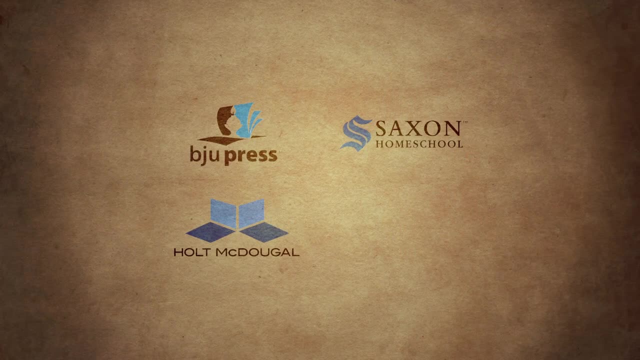 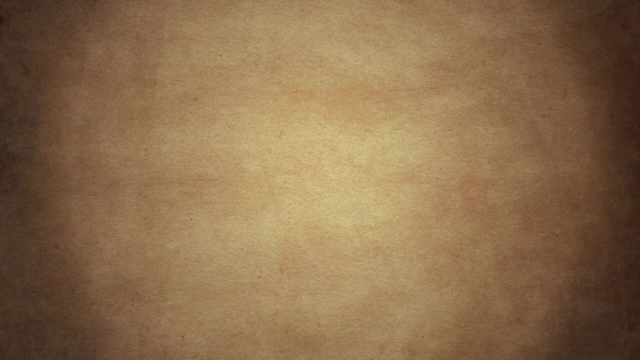 the traditional category are Bob Jones, Saxon Holt, Prentice Hall, but there are variations that would technically qualify as traditional. There are also a myriad of products that target a specific skill or skills, like four-square writing method or the adolescent literacy series, and these provide instruction and 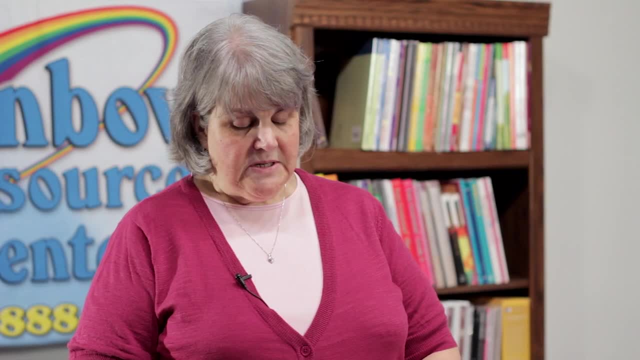 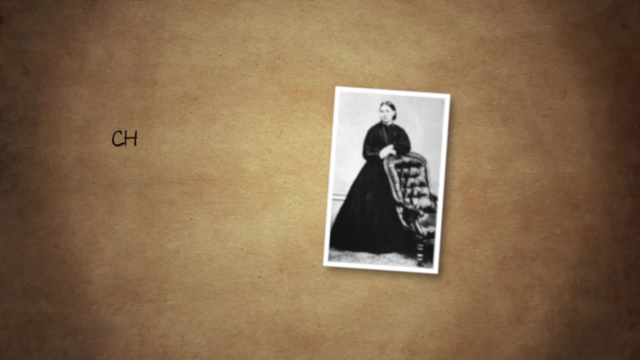